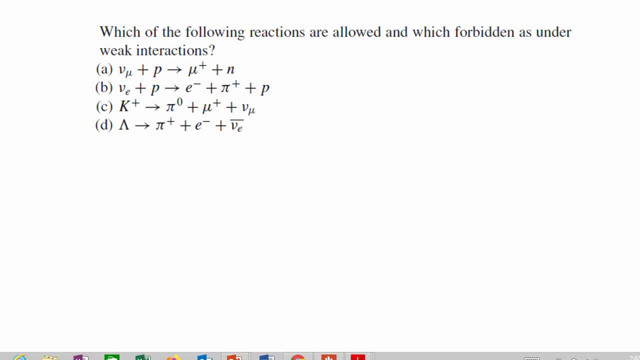 Assalamu alaikum and hi. in this video we're gonna be deciding whether a reaction is allowed or forbidden. The reaction is under weak interactions, which is radioactive decay. It just decays by itself. It has to do a lot with lepton. 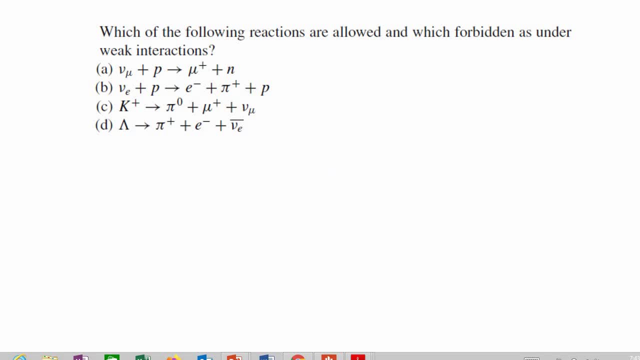 numbers, because when a particle decay, it will produce leptons. It doesn't matter if it's electron or muon or tau or electron neutrino. Let's take a look at this acronym for leptons. Do you still remember It's EMT and my text E for 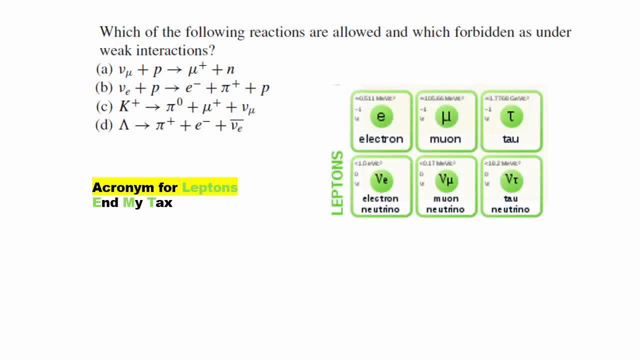 electron, M for muon and T for tau, And the other things are the electron-neutrino, muon-neutrino and tau-neutrino. Let's take a look at the charges. Electron, muon and tau has negative 1 charge and electron-neutrino, muon-neutrino and tau-neutrino. 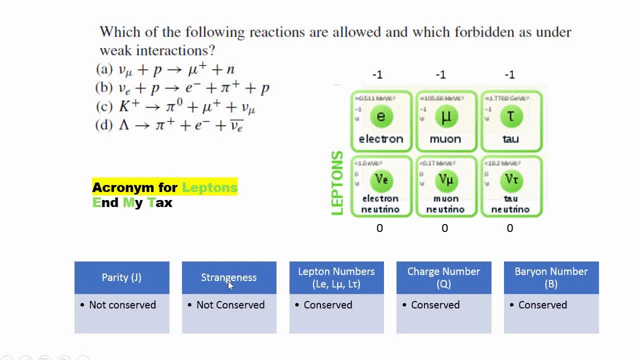 has 0 charge When we're talking about weak interactions. the strangeness is the parity is not consistent, But the lepton numbers, charge number and baryon number is conserved Every time we want to decide whether the reaction is allowed or not. you're going. 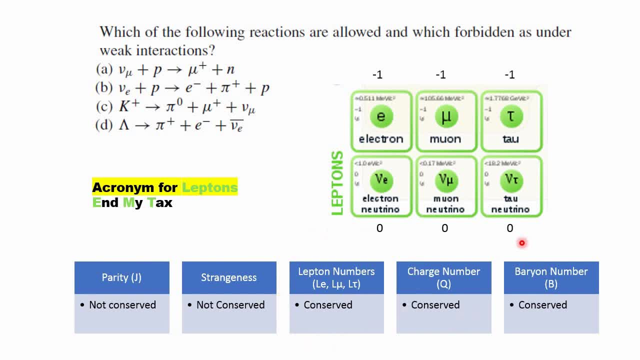 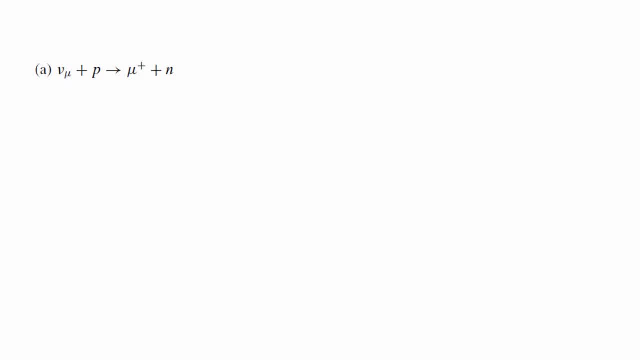 to calculate the lepton numbers, the charge numbers and the baryon numbers. Now let's take a look at the question. This is the decay of a proton to become neutron. It releases muon and muon-neutrino. For this, let's take a look. 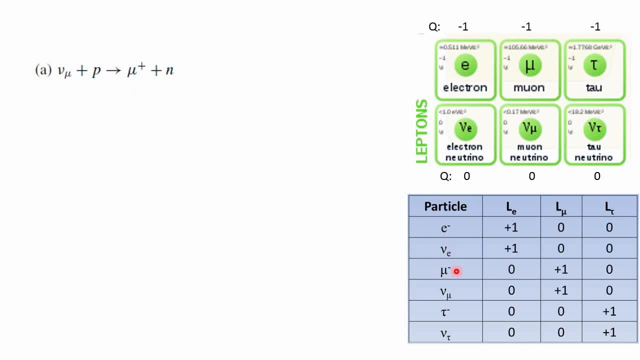 at this table. here It's all about muon, So we're gonna just see muon-neutrino. only If that muon is negatively charged, the muon number is 1. If the muon-neutrino has no bar on it, it has one muon number. First let's take a look at the lepton-electron. 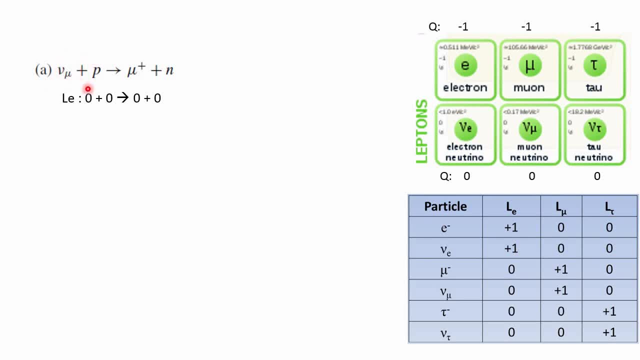 number. It has 0 electron here, so this process doesn't involve with electrons. So you can just safely write 0 here. Lepton number of electron is conserved. There's no problem with it. Next we're gonna take a look at the muon. This: 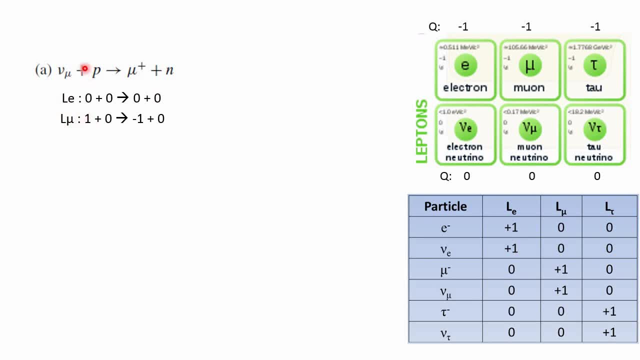 has one muon-neutrino, so the number is 1, plus proton has no muon at all, so it's 0.. And if you see here it's positively charged muon. The muon appears in the natural state. 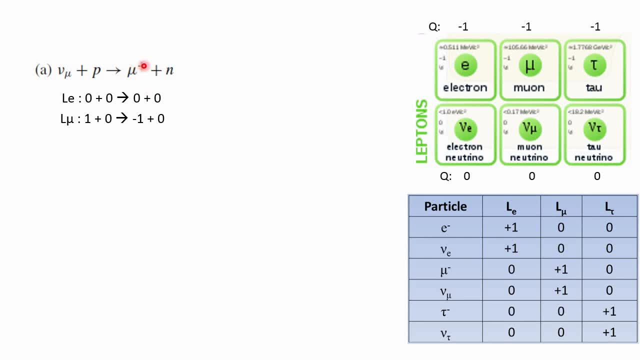 is negatively charged, but this one is positive muon, so it is an anti-muon. It is opposite from 1, so it's negative 1 plus 0.. Let's take a look at the tau number. It has no tau here. 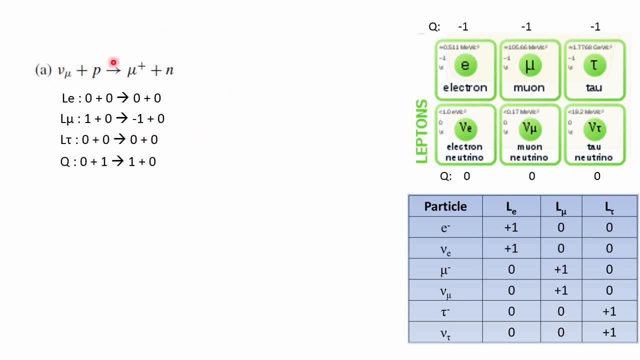 so everything must be 0, no problem. Then let's take a look at the charge. Muon-neutrino has 0 charge, So you write 0 here. and proton? we all know that proton has positive 1 charge. Muon is negative 1 charge, but anti-muon is positive 1 charge, So charge is conserved. Baryon number Muon-neutrino is not a baryon, but proton is a baryon and neutron is also. 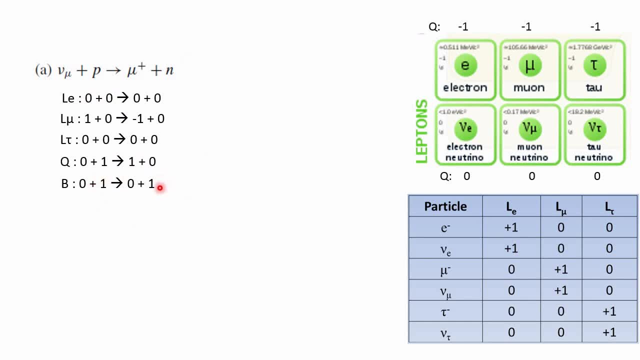 a baryon. so this must be 1 and 1 here. So the reaction is allowed or not allowed. so not, I'm gonna give you time to think. Have you decided whether this reaction is allowed or not? Yes, it is not allowed. It is forbidden because the lepton 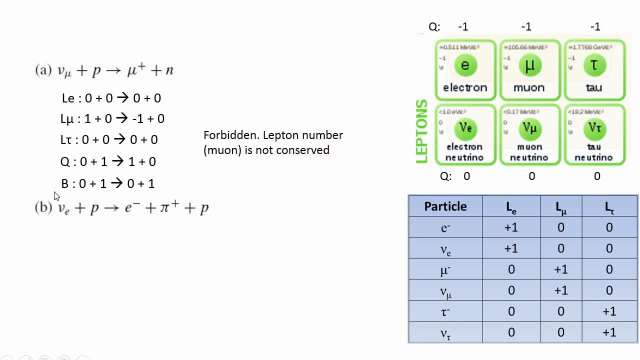 number is not conserved. Next question: This decay release one electron, so it must be involved with electron number and electron neutrino. At the left hand side there is only one electron neutrino, so the lepton number is one. proton has zero lepton number and at the right hand side, electron has one lepton number, The 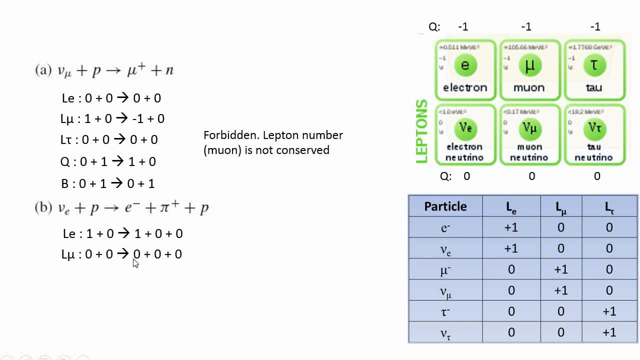 other thing is not lepton, so it's zero The muon number. This reaction doesn't involve with any muon or doesn't produce muon. so everything must be zero. So do tau. Let's take a look at the charge, The left hand side of the proton. 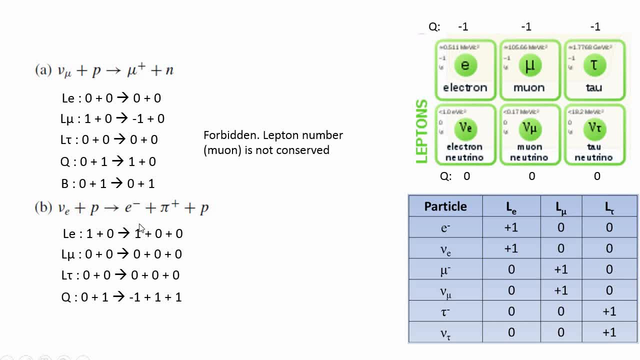 is positive, one charge and electron is negative. one positive, pi is positive, one and another, proton, is positive. one Charge is conserved: The baryon at the left hand side. there is only one baryon, which is proton, and the right hand side also has. 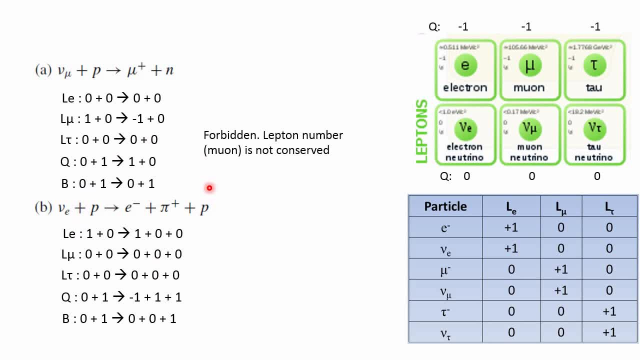 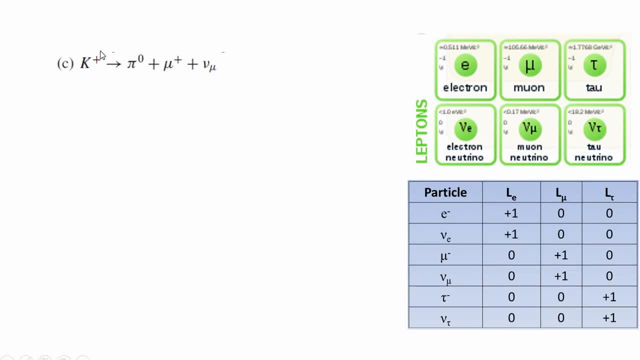 one baryon number. So baryon number is conserved, The reaction is allowed. It obeys all the leptons, baryon and charge rules. See the decay of a kaion particle. Take a look at every single product produced by this decay. It involves one. 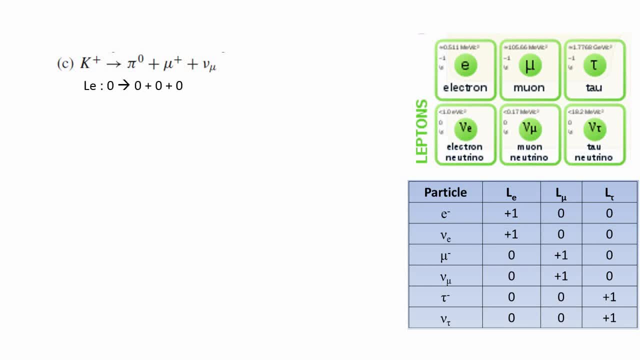 particle. There is only one particle, So electron number is zero. muon left-hand side: zero right hand side. This is an anti muon, So the lepton number is negative one. If it is negatively charged, the lepton number becomes positive one, but in this case it's positively charged. 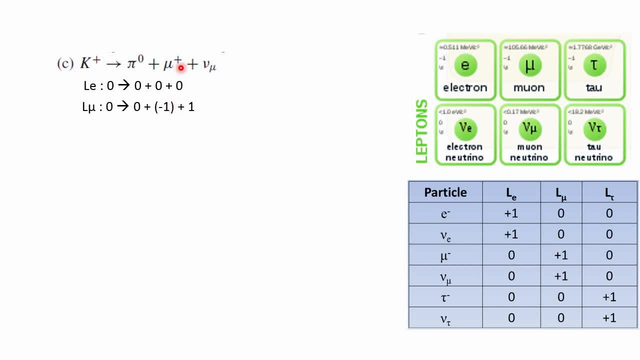 It is an anti muon, So the number is negative one and muon neutrino positive one. Tau is zero. Kaion has positive one charge. Muon is a negatively charged If it's at its natural state, but in this case it is an anti-moron, so it has positive one charge and 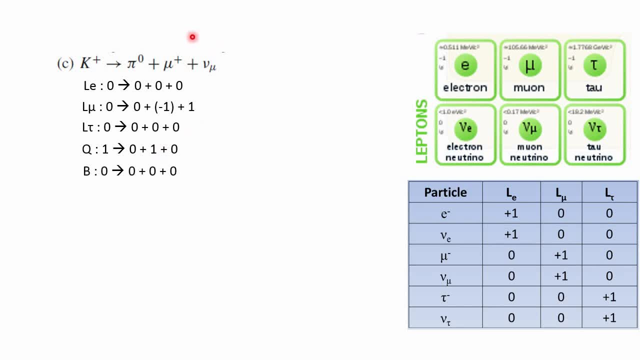 moron neutrino has zero charge baryon. there is no baryon involved in this reaction. everything must be zero. so the reaction is allowed. it obeys all the lepton baryon and charge rules. next, the decay of a lambda particle. it releases one electron and one anti-electron neutrino lepton number. 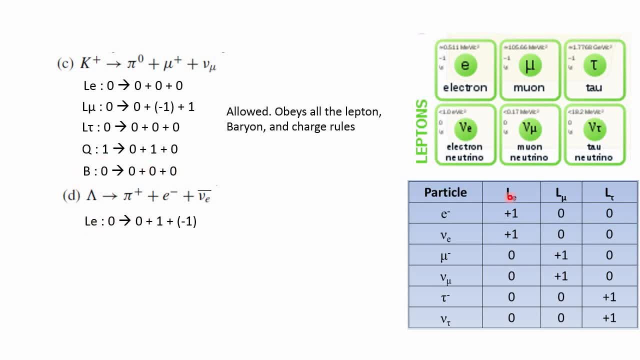 left hand side: zero. right hand side. electron negative has positive one lepton number and anti-electron neutrino has negative one lepton number. if you add up everything in the left hand side and everything at the right hand side, the answer is zero. left hand side, zero right hand. 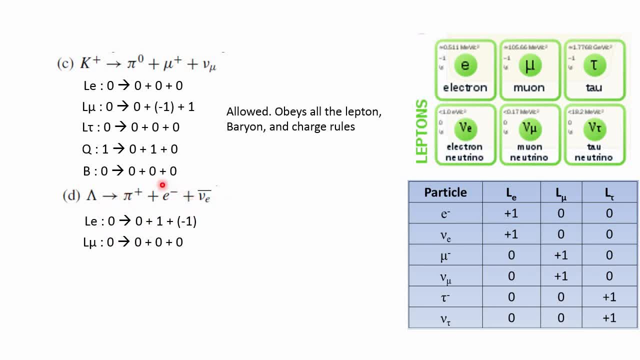 side zero, so lepton number is conserved. next the moron number. there is no moron here, so everything must be zero. tau also zero charge. lambda neutral has zero charge, moron plus has positive one charge, electron has negative one charge and anti-electron neutrino has zero charge. so if you add up all of this it yields to zero left hand. 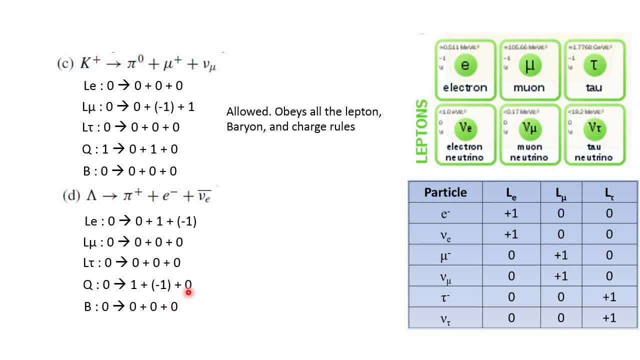 side: zero. right hand side: zero. charge is conserved. baryon number: there is no baryon involved in this reaction. baryon number is zero. the reaction is allowed because it obeys all the lepton, baryon and charge rules. the thing about the weak interaction. 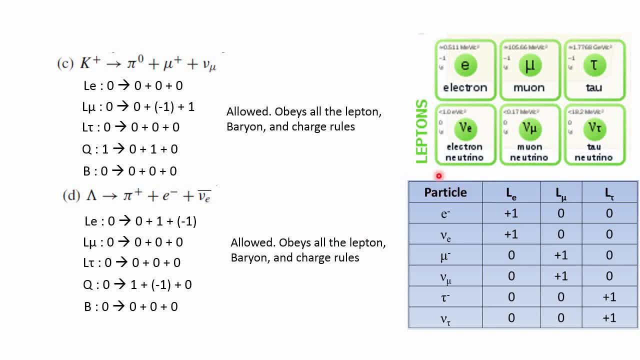 you have to remember this table because if you don't remember this table, at least know what's going on in these reactions. and you have to remember all the charges of the lepton because you want to answer the question real fast, you don't want to waste your time thinking. 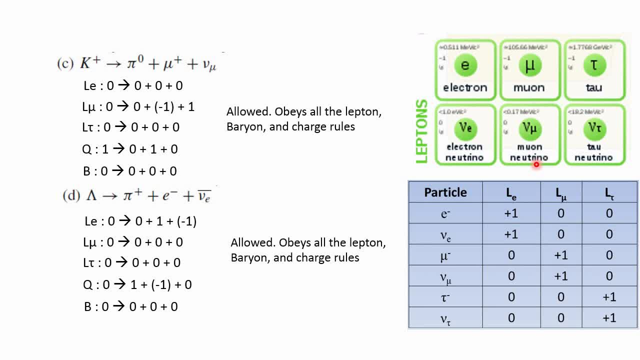 about? what is the charge, what is the characteristics? you want to straight away decide whether the reaction is allowed or not. see you guys in the next videos.